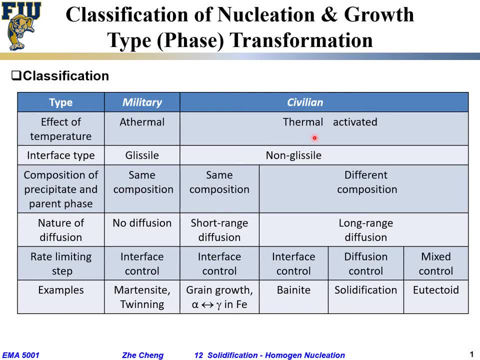 the temperature. quite often it, the transition goes faster. military is not really a temperature driven, it's not. you don't see a dramatic effect. I will put it that way. you don't see a dramatic effect from temperature on the speed or the rate of transformation. and then in terms of composition, in this phase, 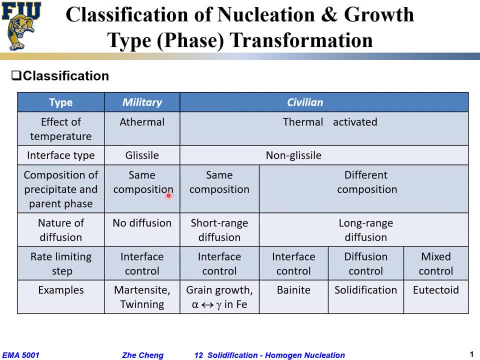 transformation for military phase. types of phase transformation, that's the new phase versus the matrix or the host of phase. they have the still very often have the same composition. so which means before and after the phase transformation the two phases quite often have the exact same composition. then you ask me what would change if the composition is changed? it's: 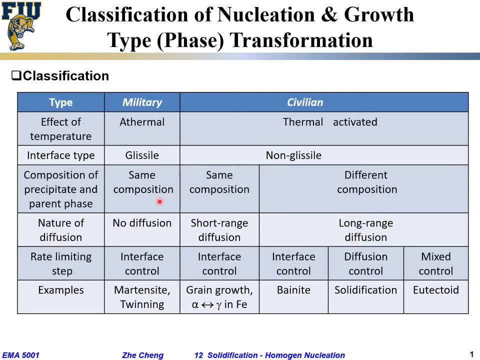 the same. what would change? well, the crystal structure may still change, makes sense. lattice parameter may change, but the composition chemically, from a atomic point of view, how many one atom A, how many atom B, they remain the same. we'll talk about this. 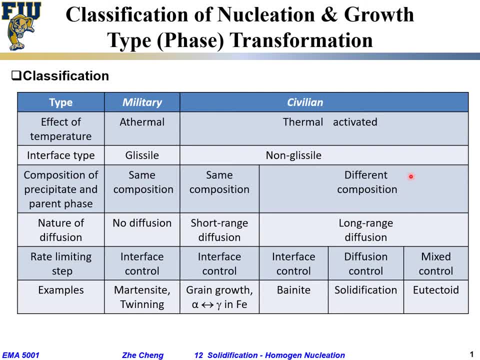 but for civilians, there are two types. the majority of them involve different composition, but there are also some that remain in the same composition. okay, and in terms of the nature of diffusion in this process, diffusion again is mass transport at atomic scale, random motion. 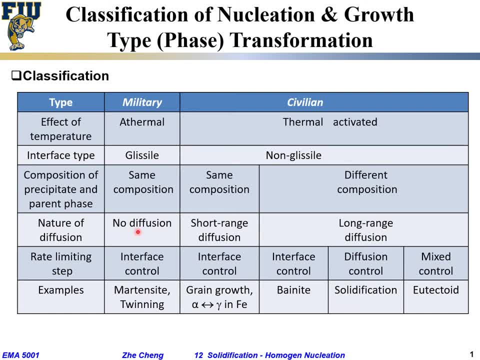 due to this and for the military types of its transformation, believe it or not, they do not involve diffusion, because it's not a random process. all the atoms would move at the same time, in the same direction, for the same speed. that's not diffusion. diffusion is what the atoms move. 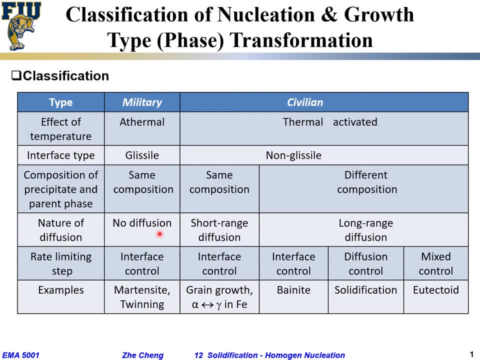 pretty much randomly. you cannot predict how individual atoms move, which direction they go. you cannot at all. so, civilians, there will be diffusion, depending on whether it's short range or long range. long range means across many, many grains. short range means kind of within a few grains. okay, and then. 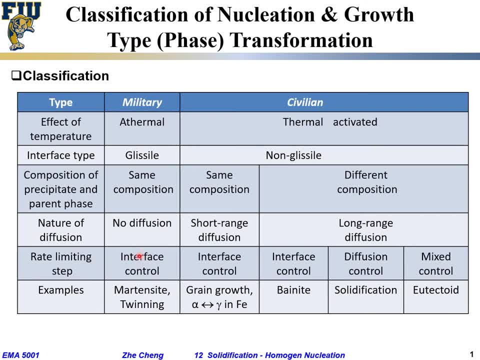 rate limiting step. okay, because military, they don't involve diffusion, so typically they would be so-called interface control or reaction control. in comparison for civilians, some of them would be remain as reaction control, which means diffusion can be fast, which means all. 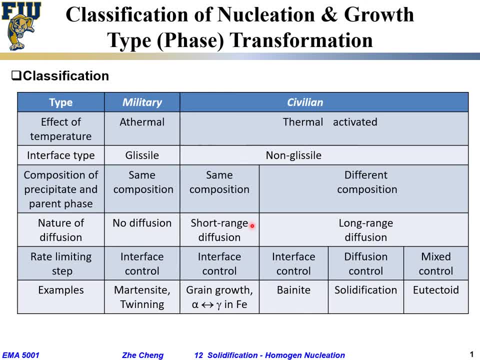 put another way, diffusion is very short range. short range, which means the time for diffusion would be long or short. short range means that square root of dt is a very small number. then i don't need a long t right. so in those cases it quite often would be so-called reaction, or 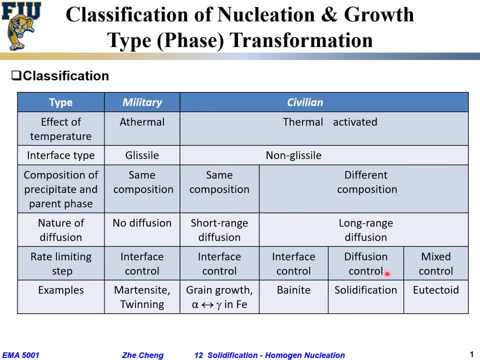 interfacial control. but for the others there can be so-called diffusion control or mixed control, reaction control and diffusion control. and we have some examples: the so-called twinning or martensite. we'll talk about that later. martensite phase transformation would be for military types. 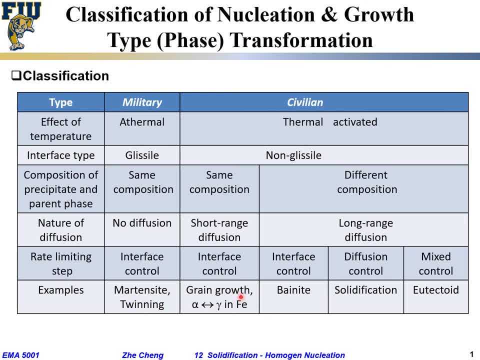 of phase transformation. well, civilians, we have the green girls. green girls, you think kind of same phase. well, one region gets larger. alpha to gamma phase transformation in iron: same composition. right, it's both iron, both iron, but from. 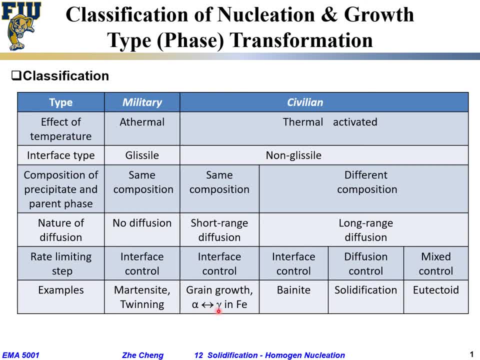 alpha phase to gamma phase, from bcc to fcc. that is a change in crystal structure and a change in lattice parameter. you don't need diffusion because composition doesn't really change. okay, in those cases it would be so-called interface control. but for some other solidification 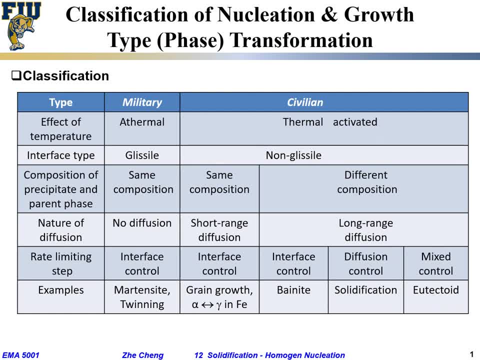 eutectic phase transformation. they all involve diffusion, and we'll talk about them later. so 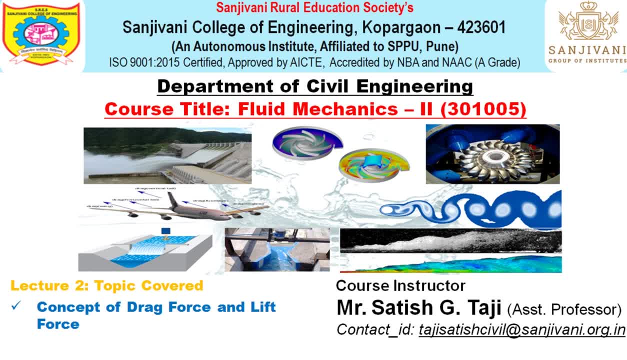 Hello everyone. hope you all are doing well, taking care of yourself as well as your family. This is our second lecture on the course titled Fluid Mechanics 2.. In the previous lecture we have discussed introduction to the submerged body. In this lecture we are going to discuss